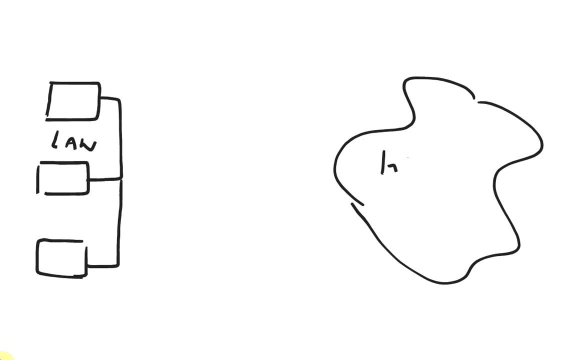 should be like Jesus. it has been converted to the real world, etc. so now let us explore in a lang 불공사, to stop in a language. using line two. we do have a few suicid banana into it. so internet, and we would like to access the internet in such a way that our LAN is secured. 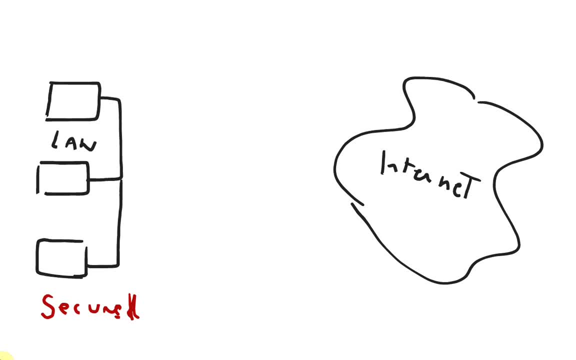 So no hacker can access our information or they may not be able to do harm to us. So for that purpose we would be needing a kind of a software or a hardware that sits between our LAN and our internet. Okay, LAN is, in this case is, the internal network and internet is the external network. 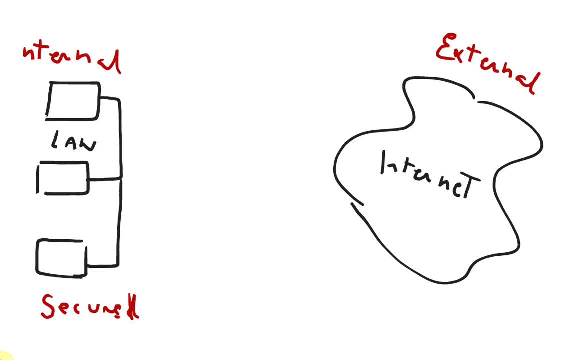 So we would like a piece of software or hardware, or combination of software and hardware, which can make us secure, and that is the function of a firewall. So we would put a firewall software or hardware In between our internal network and the external network. That external network can be internet or extranet or any kind of a LAN. 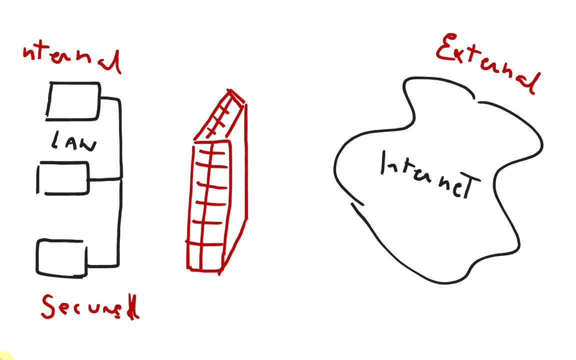 So the function of a firewall is to secure our network, and how does it do so? It checks the data packets. As we have already discussed that, the packet, that the traffic on the internet or data on the internet travels in the form of packets. So whenever some packets are coming inside our network from internet, then it is the function. 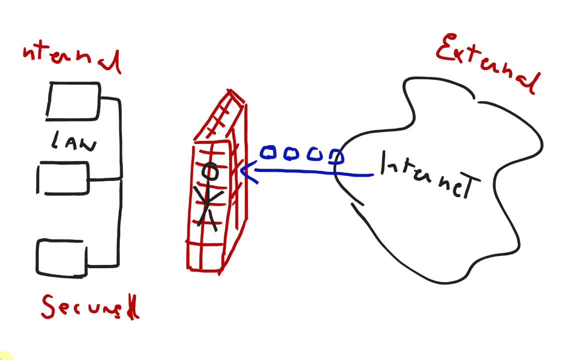 of a firewall to inspect them, to check them. Okay, Okay, So if the firewall decides that those packets are okay, then those packets are received on our LAN And the firewall does so based on the predefined set of rules. So as network administrators, we can define the rules based on which the traffic can come. 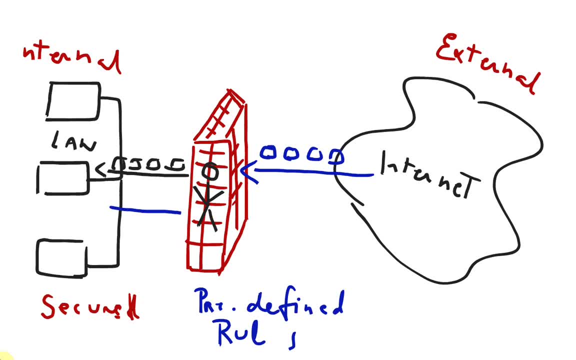 into our system or even it when it is going out. So when we are sending packets to the internet, then the firewall can also check if those packets are okay, if they meet the predefined rules, and if they do, then the firewall sends those packets to the internet. 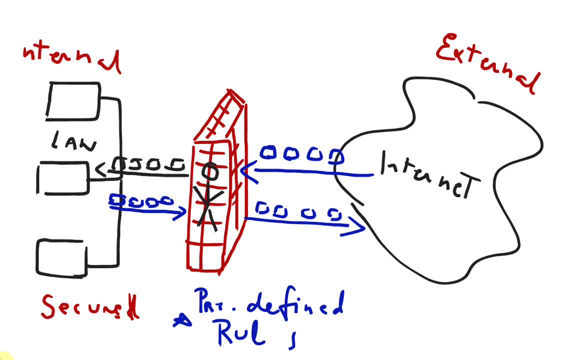 But if they don't, Then the firewall. The firewall would silently drop that packet and sends an error report to the sending PC, And that is also in the case of the traffic coming in from the internet. The firewall checks if that packet is okay. 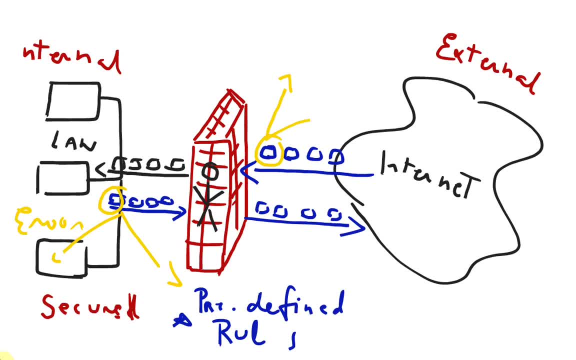 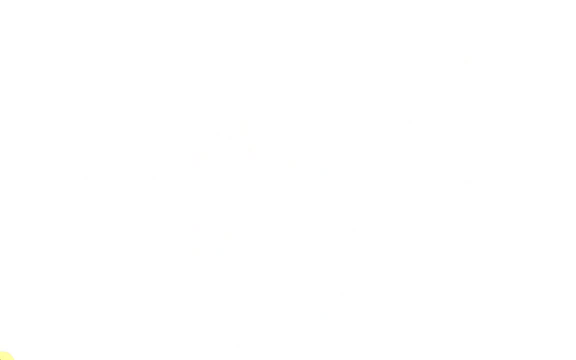 If it's not, then it drops that packet and sends the error report to the sending PC. Okay, Okay, So this is the function of a simple firewall And, as I have already told you that there can be two kinds of firewalls, One is only software based firewalls. 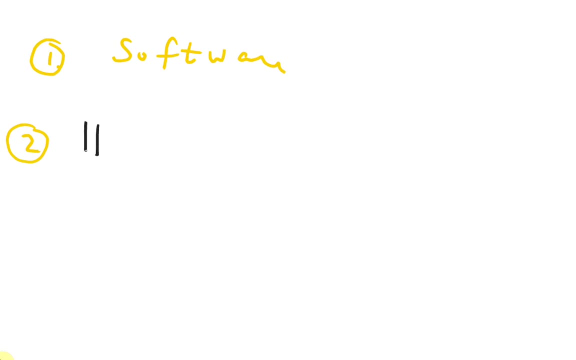 And the other one is the hardware based SAR firewalls. So at In our homes, Usually In our personal computers, we use software based firewalls, And if we have got a bigger network, for example in an office, then we use hardware based firewalls. 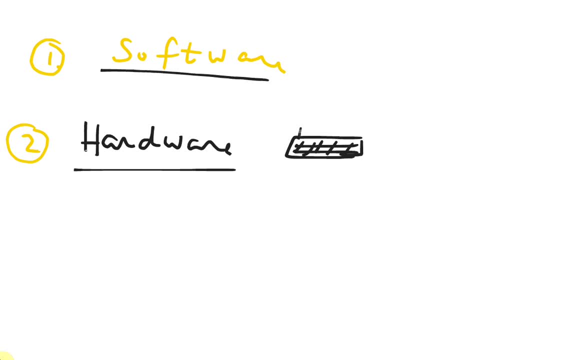 And those firewalls have got software component which checks that The invalid packets Or traffic cannot come Or go out from our system. And today's routers can also act as a firewall. So there is a built in firewall in today's routers. 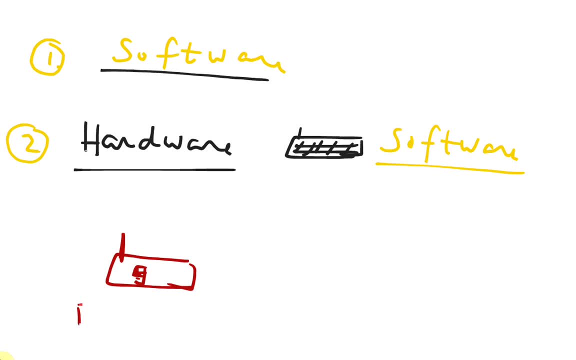 In most of the routers. So these routers can act as the routers and also as the firewalls And, conversely, The firewalls Can also perform The routing Function. So They can, We can buy a firewall and we can use them as a router. 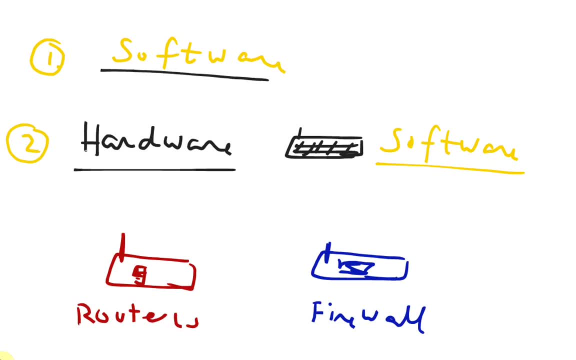 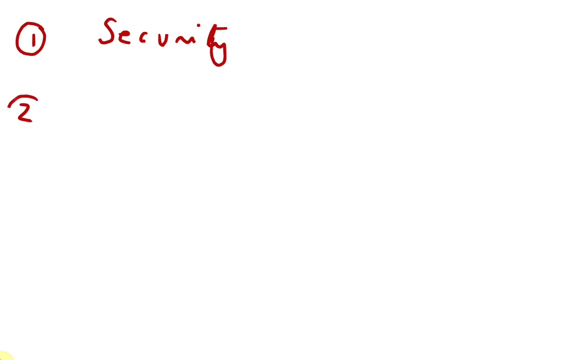 Also And And The purpose. Now we will discuss Two main Purposes of the firewall. One, as you have already discussed, is That we use firewalls for the Security reasons, To secure our network, And the second purpose of the firewalls. 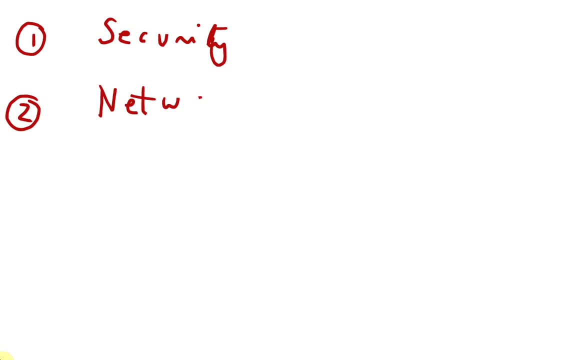 Is the network administration In the firewalls. We can. We can block the ports Or the protocols So that Those ports Or protocols Can not be used, For example If, As a network administrator, We would Like. 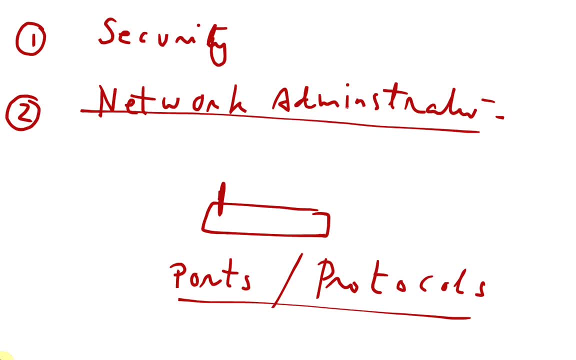 That Nobody can Use The FTP port Or the FTP protocol Or data being transferred through FTP protocol Or through Telnet, Then We can Basically Block Those Port Protocols So that Those ports 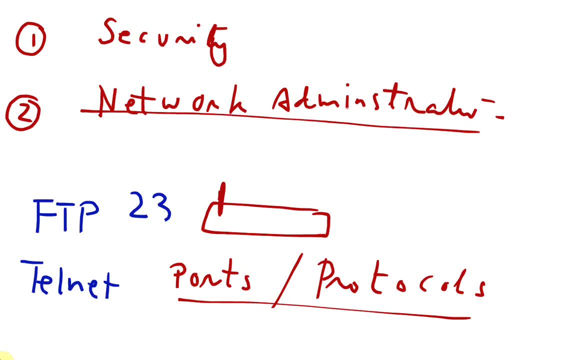 Protocols Can not be used, For example, If We Block Those Ports, And We can Also, As network administrators, Block Special Websites, Or We can block, For example, VoIP On our network. 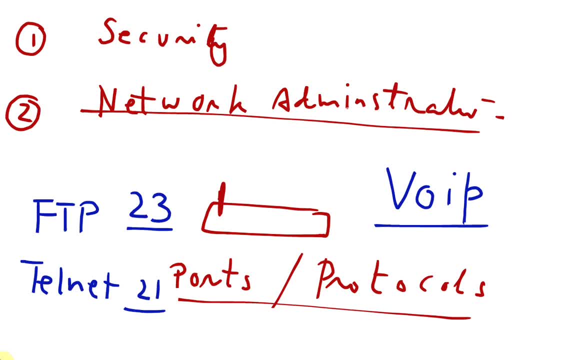 So nobody can Place IP calls On our network As network administrators, So We can Also Do that. So There are Two main purposes Of the firewall. One Is Security And Number Two